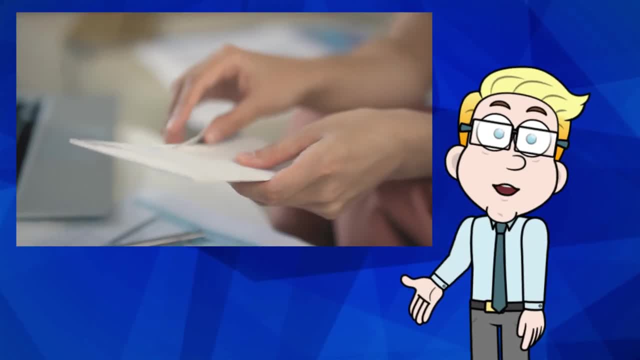 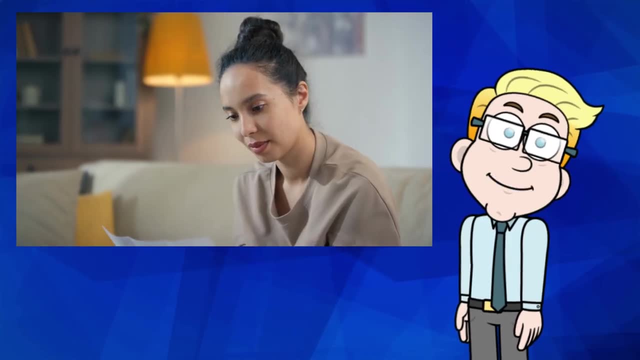 If you are employed, you may have received a paycheck with a pay stub attached. Congratulations, you got paid. If you receive a physical paycheck, the pay stub is usually attached to the check. If not, you may be able to access your pay stub information online. if 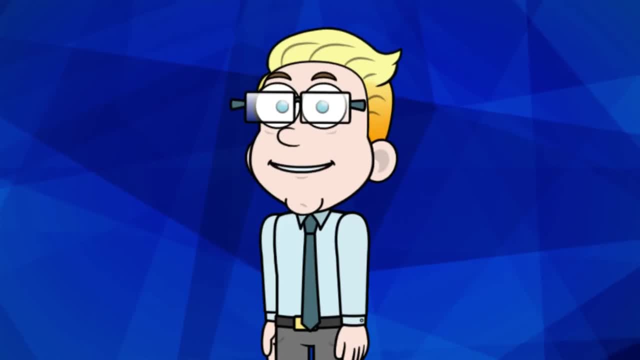 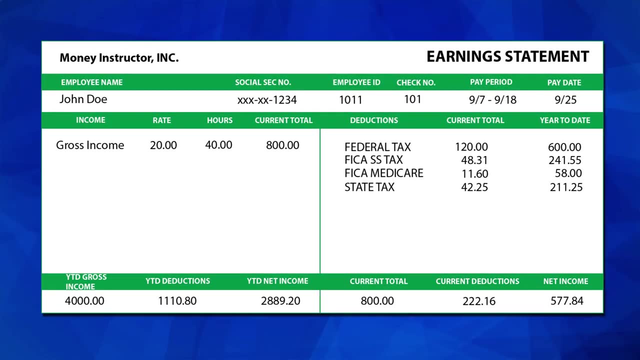 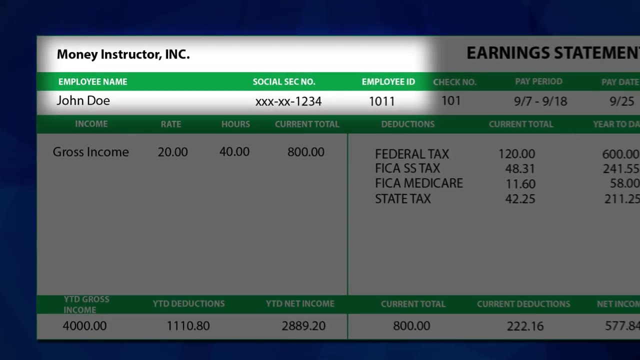 direct deposit is used by your company. Let's take a closer look at the information you need to know on your pay stub. The first thing to note is company and employee information. This section includes your company's information, also your name, employee number and related information. Next is pay period: Pay period. 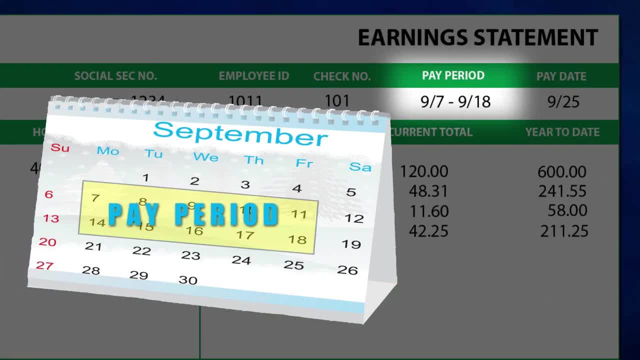 refers to the time you have worked. A bi-weekly pay schedule, for example, calculates a two-week pay period. Pay date: Pay date is the date you receive a paycheck. Many companies pay their employees on a regular basis, such as every other Friday. This would make Friday the day you receive. 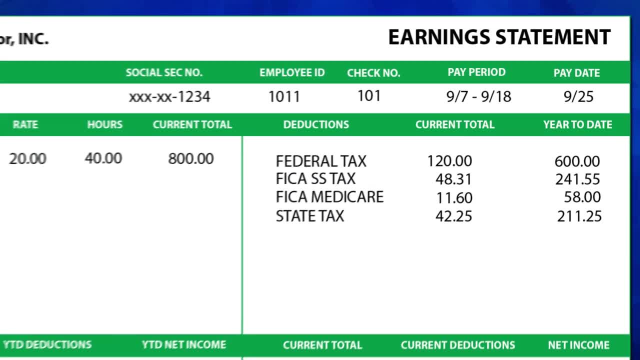 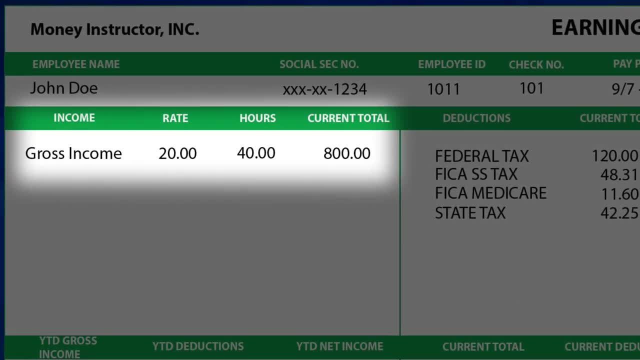 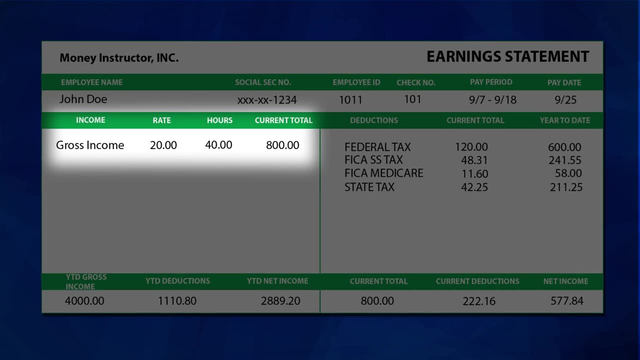 a paycheck. The next section is your gross income. This section of your pay stub shows your gross income, which is also called wages or earnings, and is a calculation of your hourly rate in your hours worked if you are an hourly employee. The total is your gross earnings, which is the amount 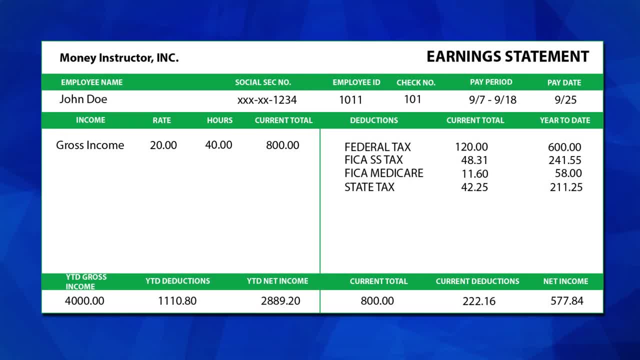 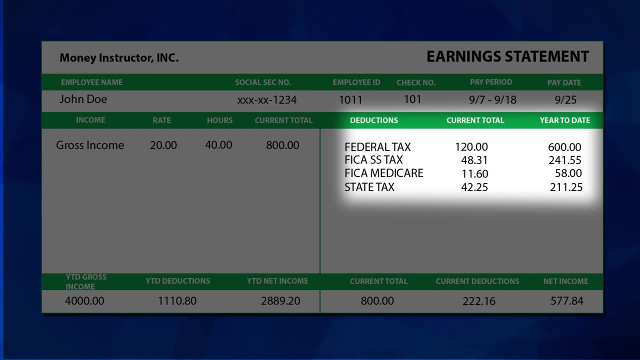 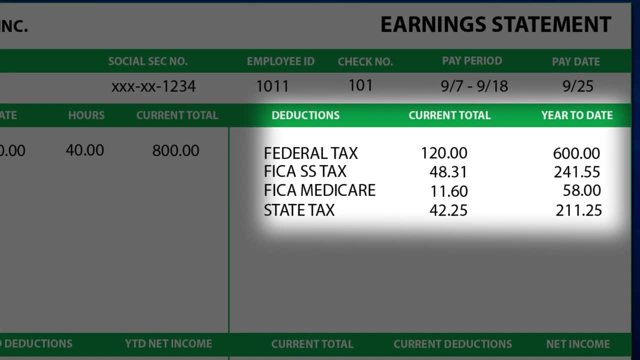 you would make before taxes and deductions. Deductions: This section contains the taxes taken from your gross earnings. The employer sends this money on behalf of the employee to the government. Federal income tax, Medicare and Social Security are the three main types of federal taxes. 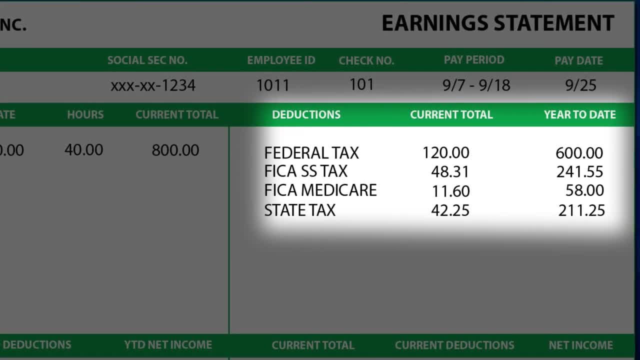 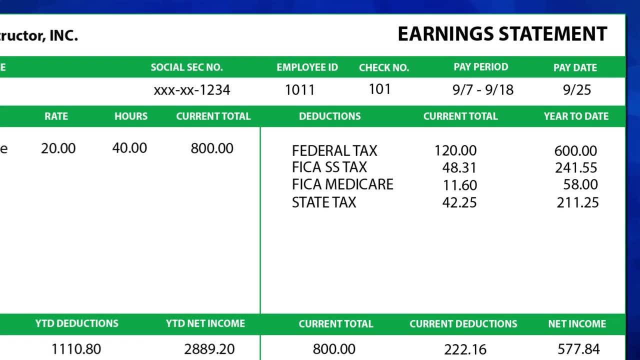 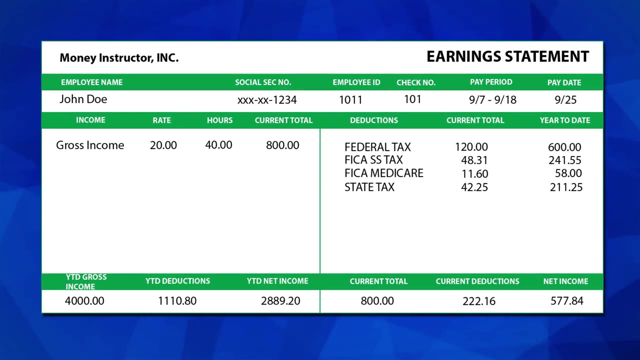 withheld from your pay. Many states also withhold their taxes. You may also have other employee deductions. This sample pay stub does not contain any employee deductions, though you may have some Employees have the option to withhold contributions for retirement funds, health savings accounts and other benefits. Next is the summary section. This is the summary. 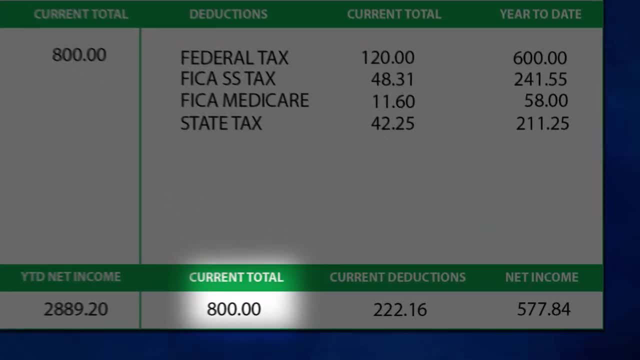 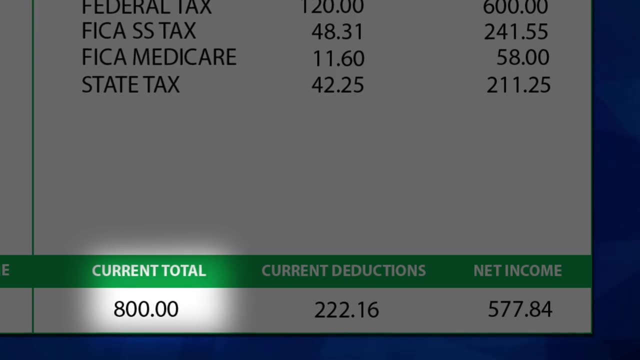 section on your pay stub. This is the summary section on your pay stub. This is the summary section on your pay stub. Here, current total is gross income or gross earnings. This number is the same gross income as we saw earlier. This is the amount you earned during this pay period before.